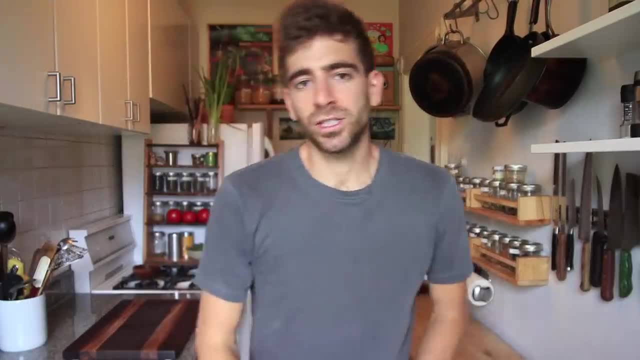 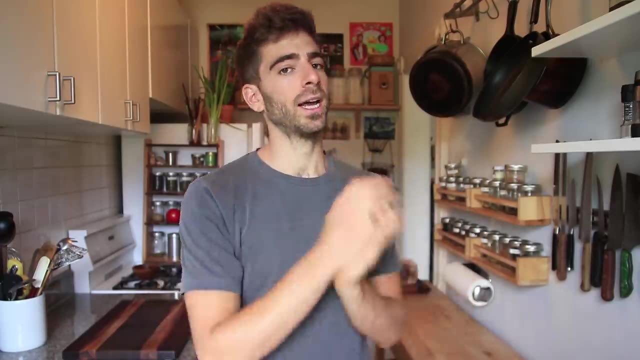 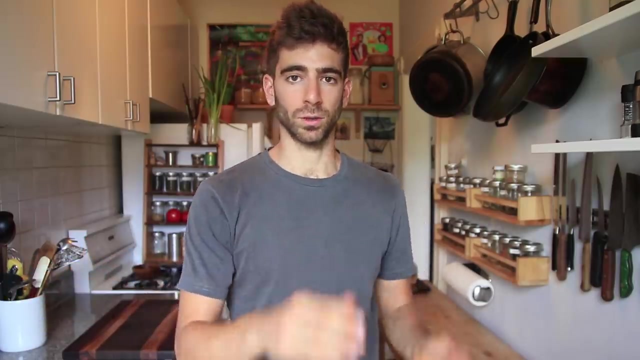 The other day I was teaching one of my friends how to cook for the first time. We were talking ground level stuff. This person did not have many skills in the kitchen, so we started off with a very basic dish and I just took them along for that journey and taught them things along the way. 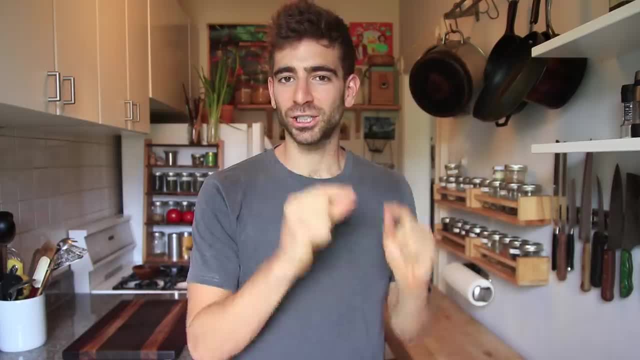 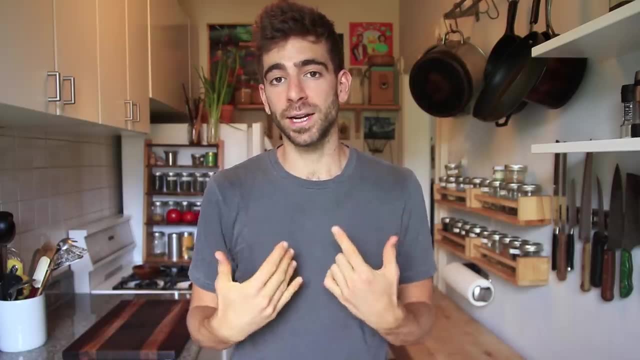 but what I was realizing was how many tips and tricks and skills you can learn from one dish. I started pointing out all these things- things that I take for granted- that can actually make you a much better cook. So that's what this series is going to be about: It's going to be breaking 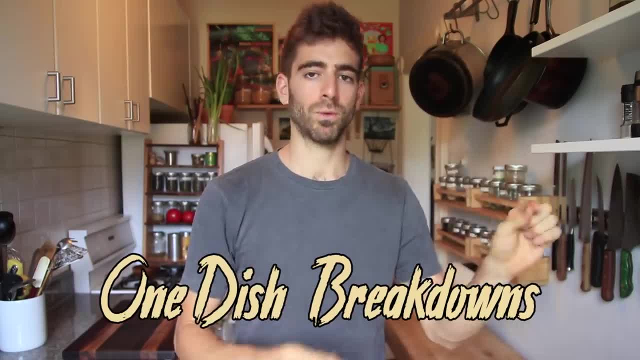 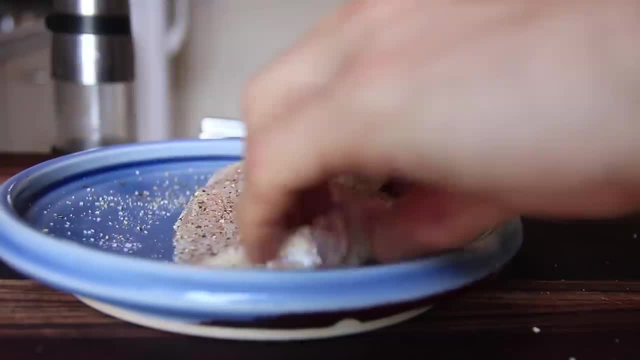 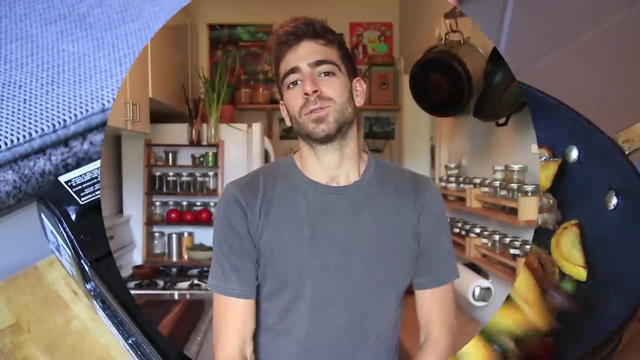 down one dish extremely in depth, going through all of the tips, all of the skills that you might not be thinking about- maybe you don't know about that- can make that dish incredible, but also can just enhance your cooking skills in general. So if you guys have been a subscriber for years, a lot 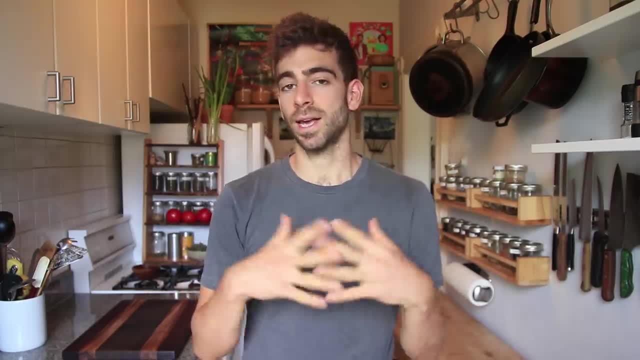 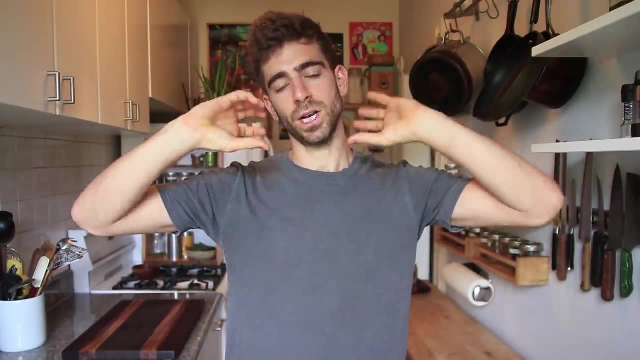 of these things might be a little too basic for you, and that is all right. That means you're already a great cook, but I know there are a ton of beginners out there and this series is going to be perfection. It is really going to take your cooking skills from that base level to the top. 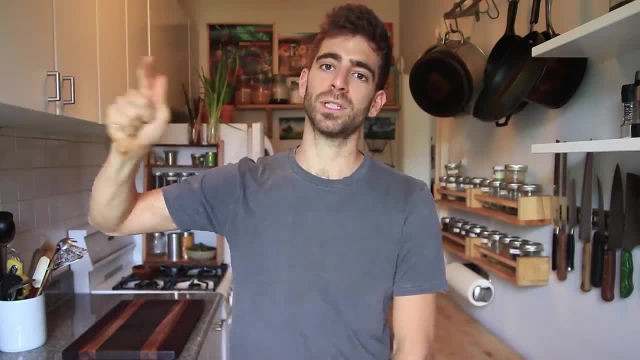 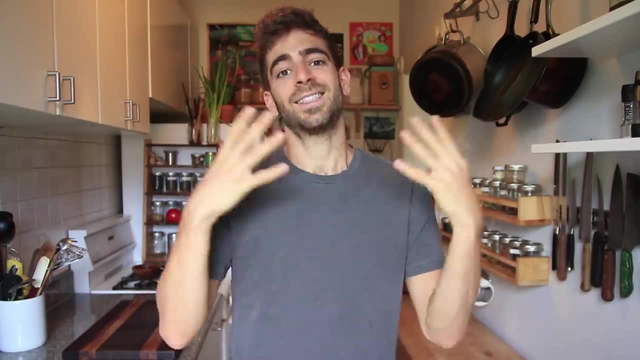 to the top notch, You'll be cooking better than the Brothers Green in no time. So the first dish we are going to start out with is one of my favorites, something I've been cooking for years. It's a stir fry, and if you can master just the stir fry with some meat or some fish, you can cook. 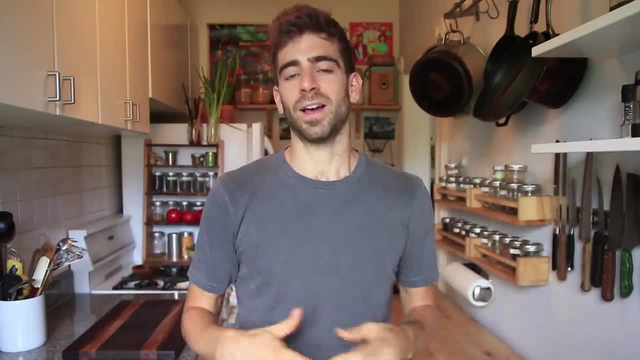 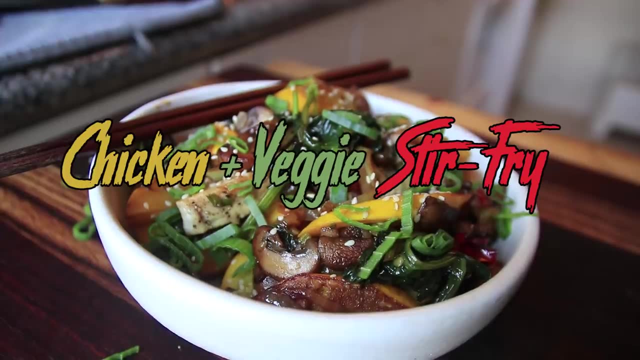 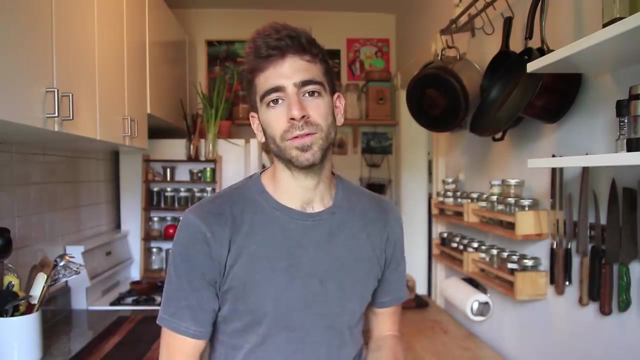 that dish for the rest of your life and probably be satisfied- at least some type of variation of it. So let's get after it. We're going to do a chicken and vegetable stir fry, because that's what I have in the fridge, but feel free to sub out the chicken for any type of meat or any type of fish, and that. 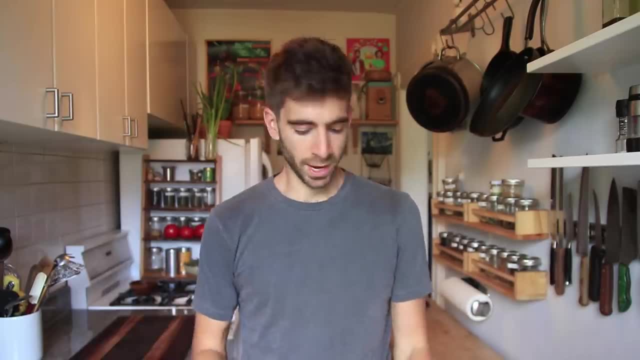 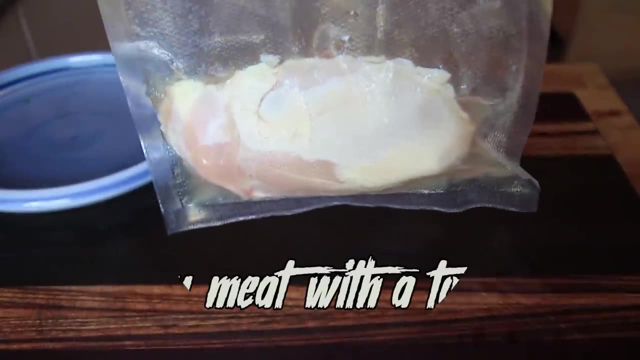 goes for the vegetables as well. You can sub those out for whatever you have. These tips are still going to work great for whatever you guys have in your fridge. Tip number one: make sure the meat is extremely dry. If you have a lot of meat in your fridge, you want to make sure that the meat is. 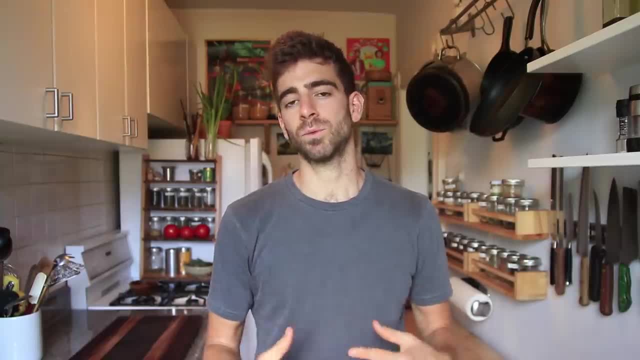 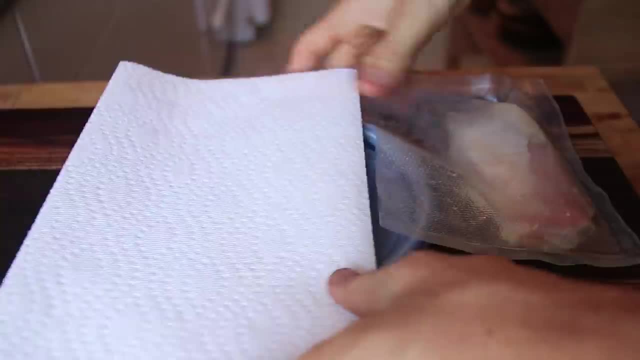 dry. You want to pat it dry with a paper towel. A lot of times, when the chicken is like sitting in a bag or whatever it comes in, it's going to have a lot of extra liquid and what's going to happen is, if you try to cook that chicken just like that, you're going to boil the chicken and that is not. 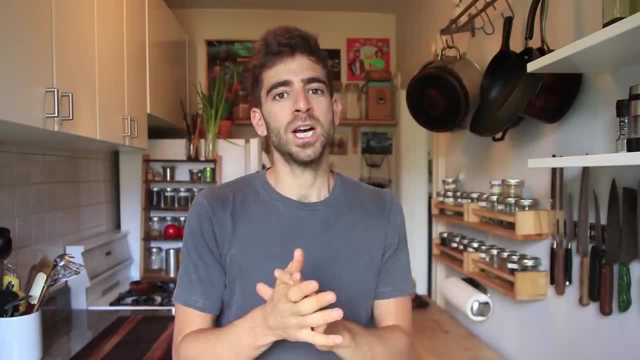 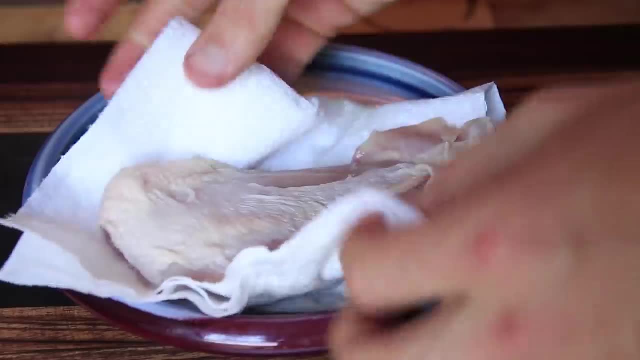 what you want, because, well, it's what you want if you're boiling chicken. but if you're actually trying to fry chicken and caramelize the skin, that's where the flavor is going to come from, and if it's wet, you're not going to get that stuff. Tip number two is evening out the chicken. 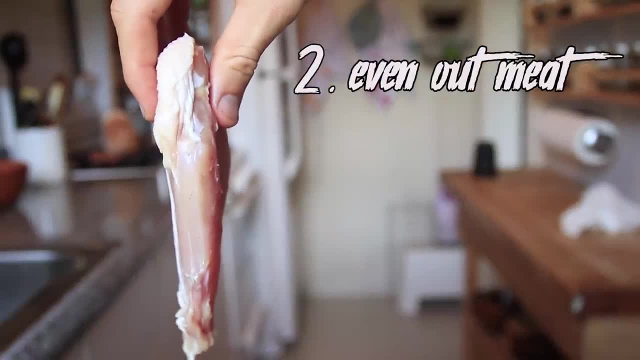 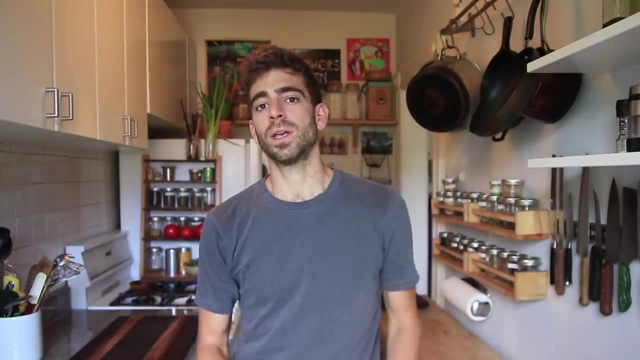 You're going to want to make sure that you've got a thick side across your meat and, as you can see, this chicken breast is uneven. We've got a thick side and a thin side, and chicken is already extremely difficult to cook because it dries out so easily. so evening out the meat is going to help. 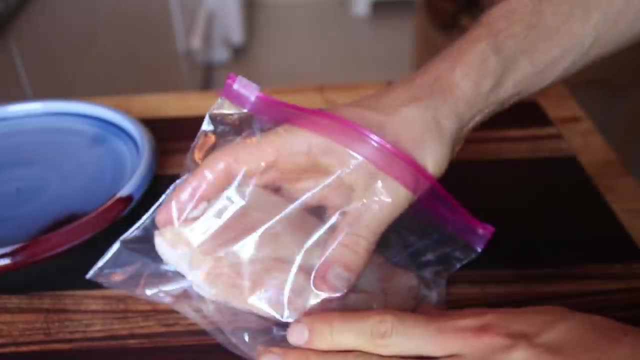 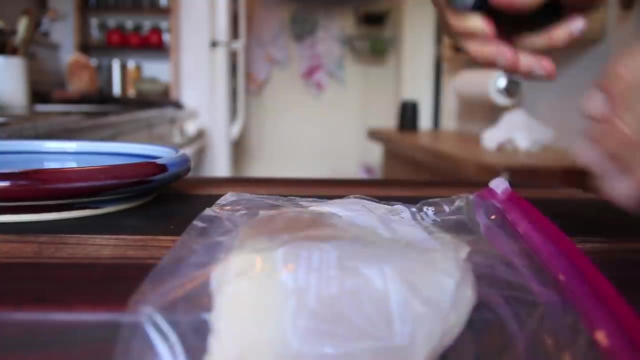 you so much. in the long run We're going to put it in a bag, something that protects it from the cutting board, and pound it out until it is nice and even so, that thick side. you can just kind of work on that until it mimics the thin side. 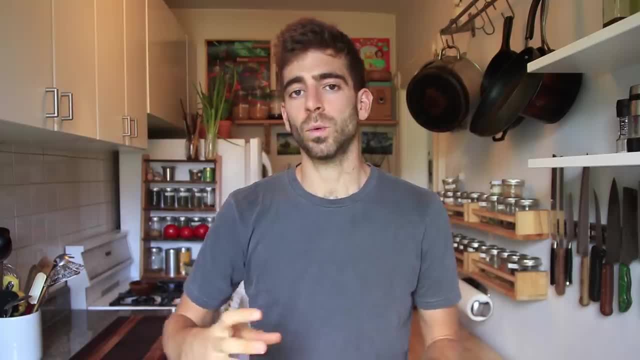 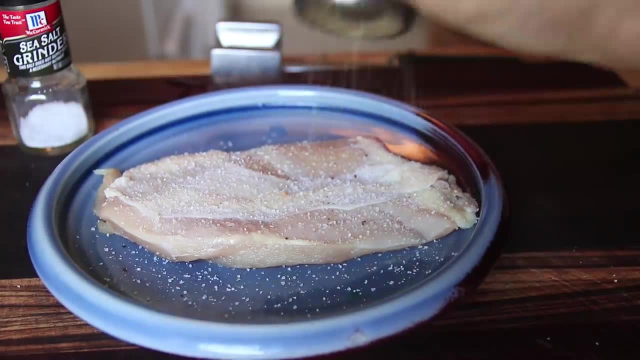 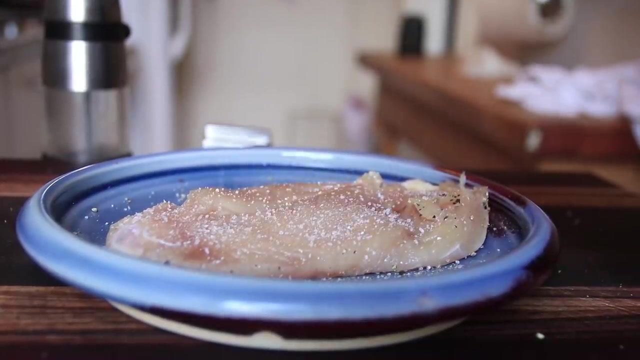 We're going to make sure that you have enough seasoning because, remember, you are seasoning just the outside of the meat and that has to carry through the entire piece. so just think about it like when you're biting into a piece of meat: the only seasoning you're going to taste is that outer. 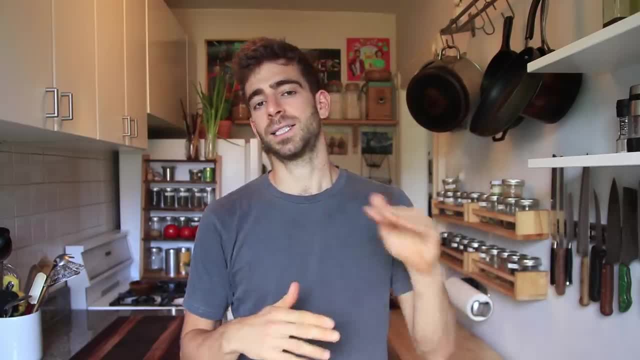 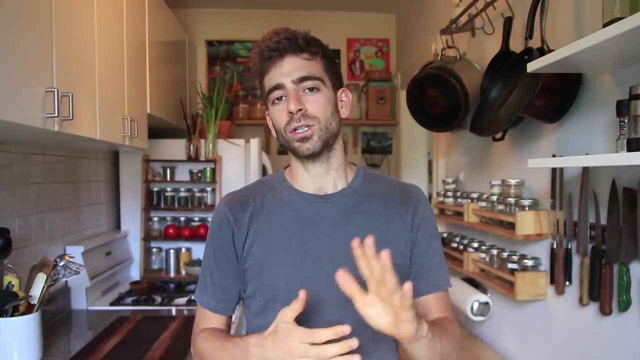 layer. If you tend to follow recipes, a lot of times they skimp on the salt and your stuff turns out under seasoned. and that is probably the easiest way to skimp on the salt- Screw up a dish. so make sure you've got enough seasoning on there to really bring out the 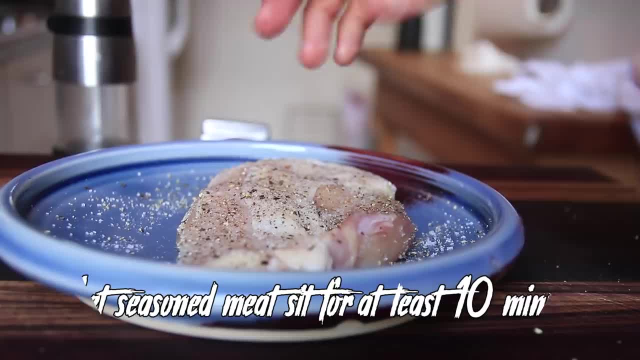 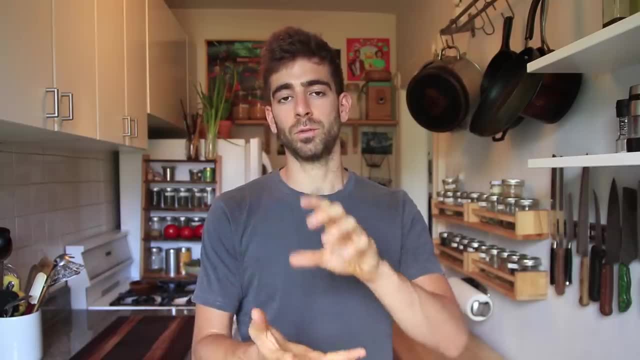 flavors. and then the next part is: just let that sit for a little bit. if you're not going to cook your meat for a little bit, just put it in the fridge let it dry out. so the salt is actually going to pull a lot of moisture out of the chicken, which is going to help with that caramelizing. 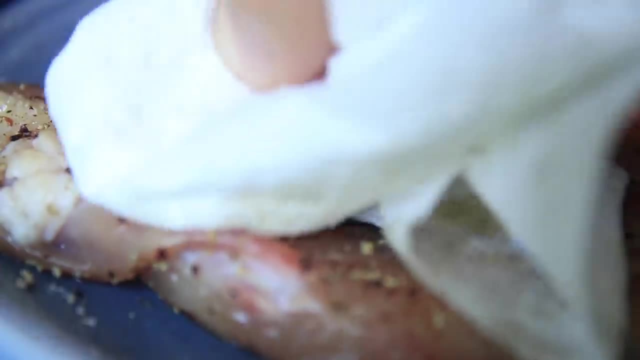 So if you just let that sit for at least 15 minutes before it goes into the pan, you'll see it's going to start pulling out that liquid and then again you're going to want to make sure that you have enough seasoning on there to really bring out the flavors. 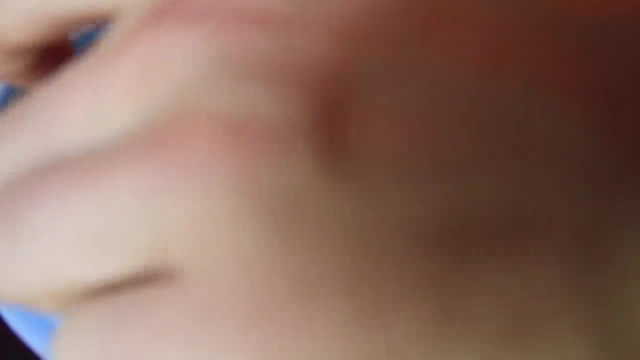 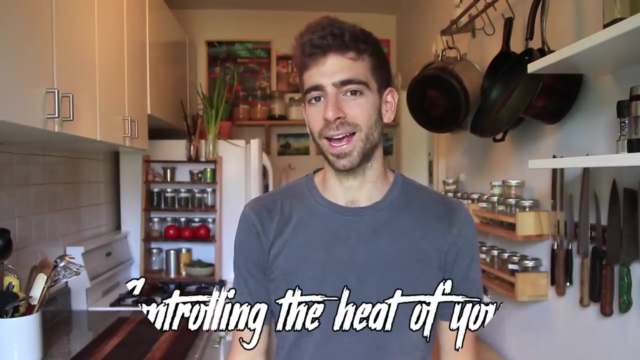 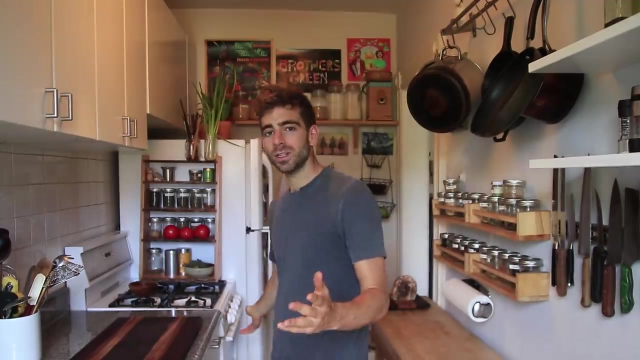 Again. just give that another pat dry and you are well on your way to crispy skin. Tip number four is controlling the heat of your pan, which seems so obvious, but I see this all the time, whether using gas or electric. there isn't just one setting. I swear, there's a ton. 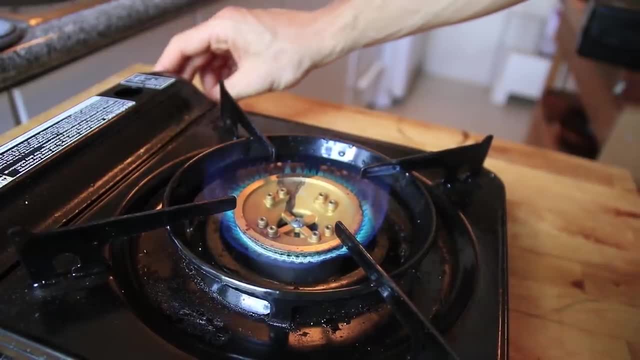 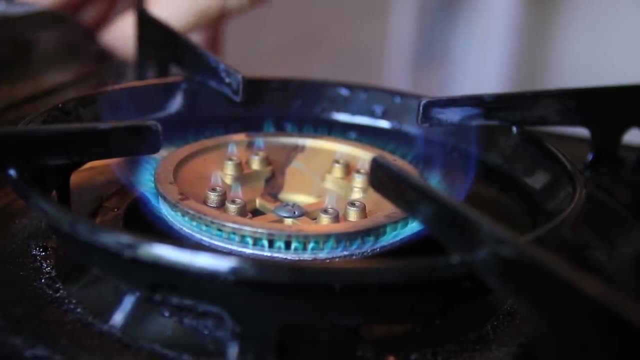 of control when it comes to the actual heat. you've got a very low simmer, you've got a medium low, you've got a medium, you've got a medium high and then you've got a high heat. so there's a whole range of heat settings and it's just something you got to get used to. but remember. 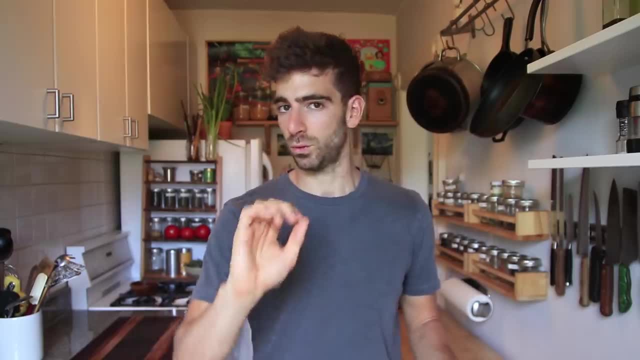 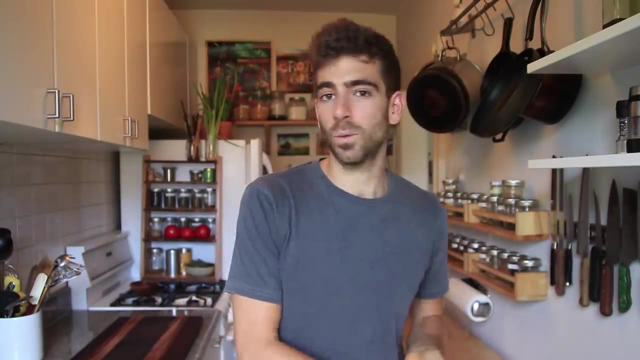 throughout your cooking process. you have the ability to control that thing. so if things get too crazy and too hot, just turn it down, and if you're not getting the action you want, just turn it up. so you are the master of your heat settings. That brings us to tip number five, which is making 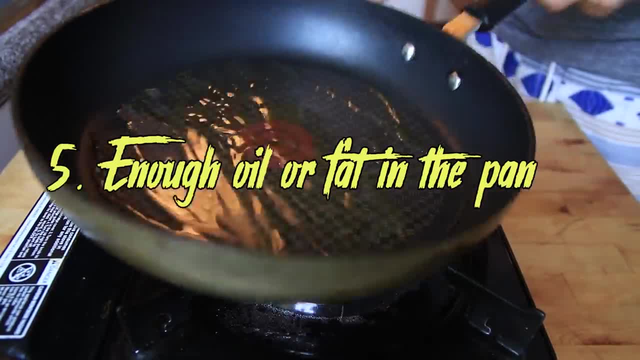 sure you've got enough lubrication in that pan so things cook properly and don't burn. Another one: I see all the time people are safe. Tip number five, which is making sure you've got enough lubrication in that pan so things cook properly and don't burn. 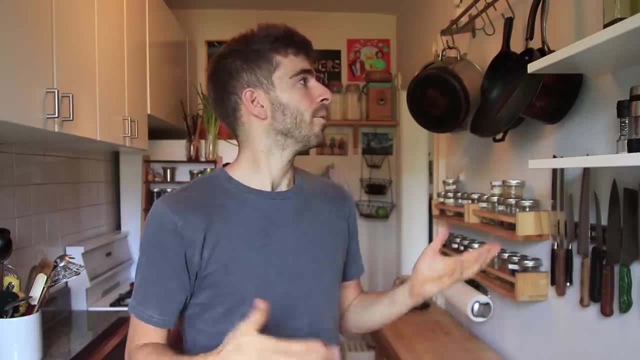 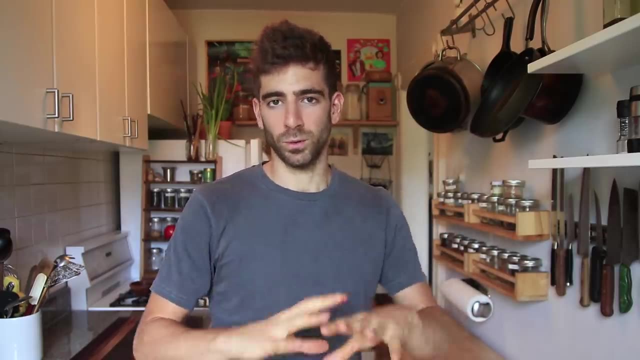 Another one. I see all the time people are safe skimping out on the oil or fat. Maybe it's health reasons. They're a little scared of it. I would say, if you're scared of using too much oil, just try to get a healthy oil which isn't going to be. 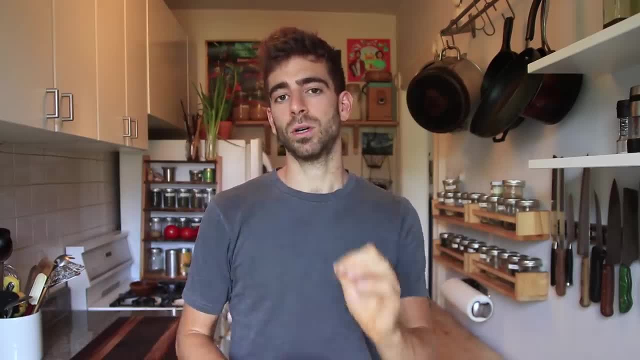 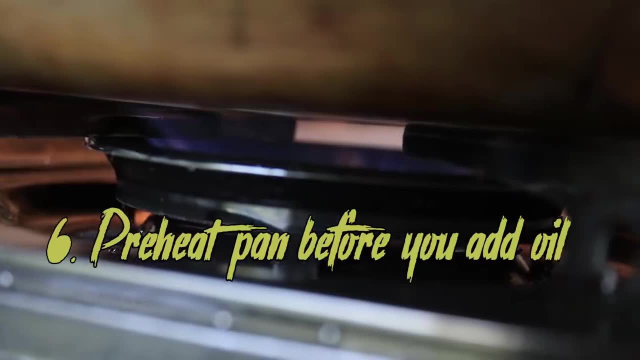 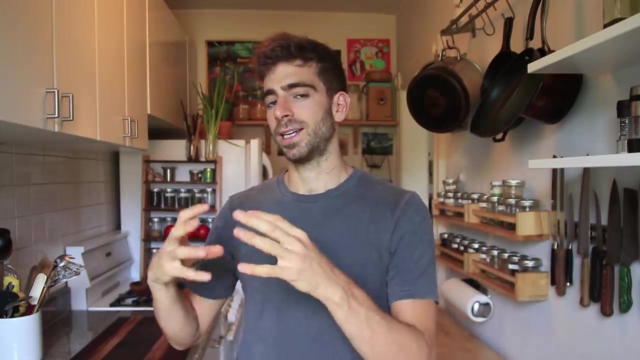 bad for you and make sure you put enough in the pan so you can cook your stuff properly. So tip number six is: make sure you heat up that pan first before you add the oil. So once it's lightly smoking, then add your oil, because if you add it earlier it's going to start to degrade as it. 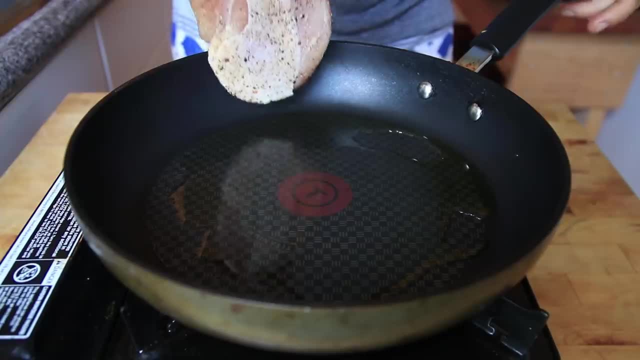 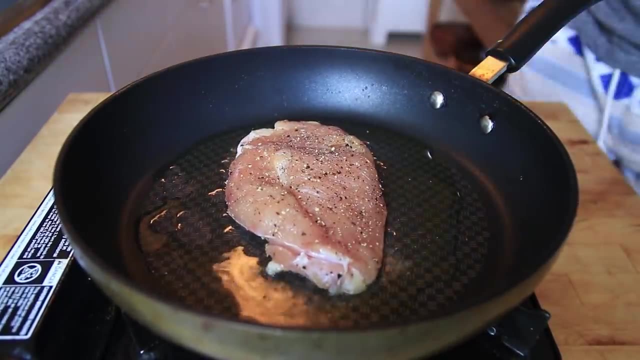 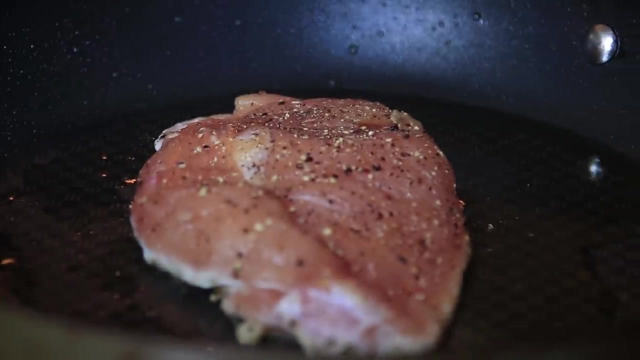 heats up, So you want the least amount of time with that oil in the pan. Now we are going to slide in that chicken and get that crispiness and we're not trying to blast this chicken away. We are trying to slowly develop the crust over time. That's why we've got that medium low heat going. 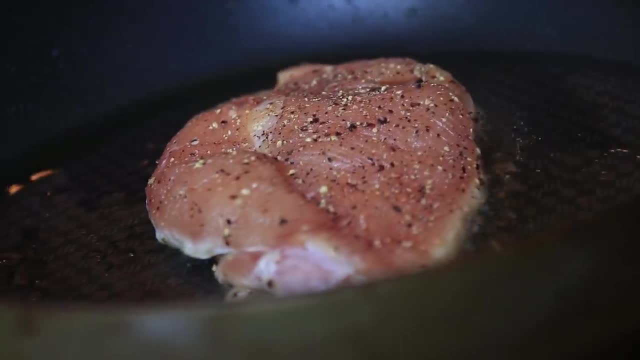 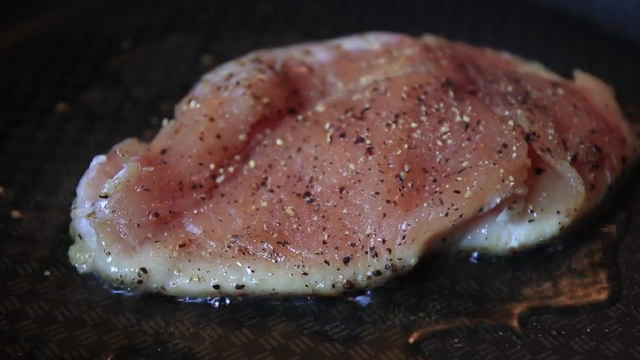 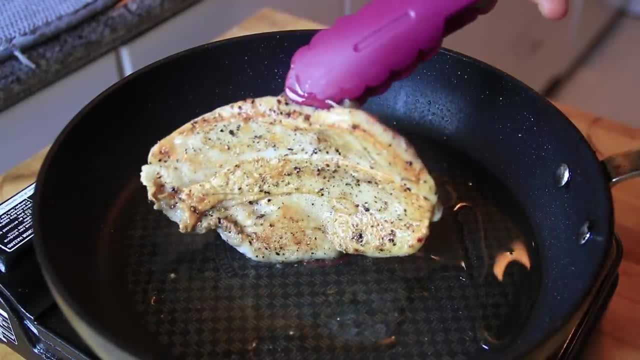 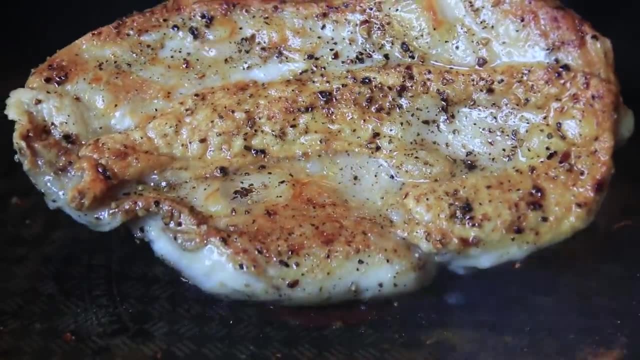 bit of oil, and I'm going to take a little bit of oil, and I'm going to take a little bit of oil, and right there, the crust is not good enough for my liking. So we put it back for another minute and then we hit our perfect caramelized point right there, Flip that chicken over and then 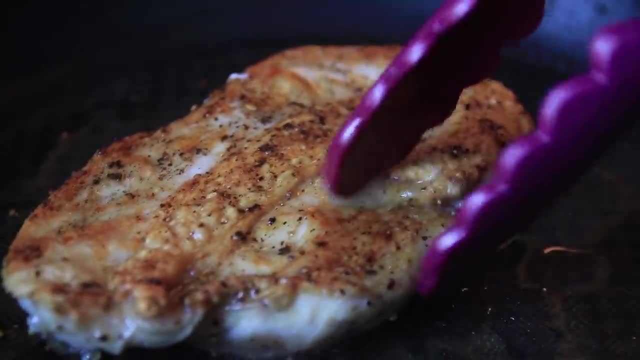 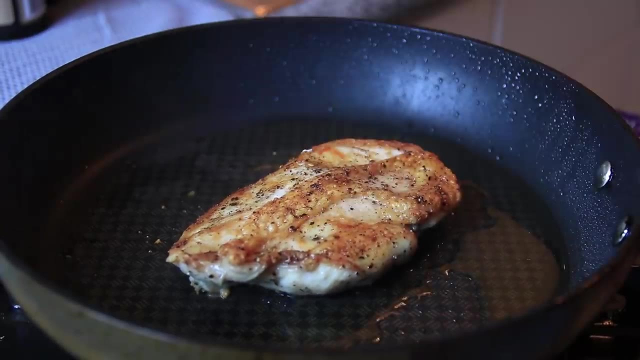 it's always going to be a little less time on the other side, So cook that side for about two to three minutes. So tip number seven: when you're feeling that chicken and it's nice and firm but it still has a little bit of give, you can pull it and you don't have to cook it completely through, especially. 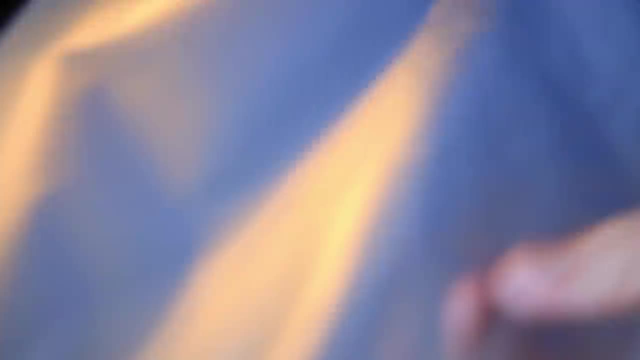 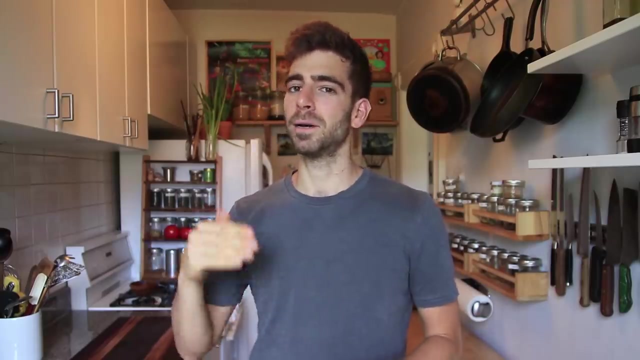 with chicken breast because it dries out so early. So I would recommend pulling it just a little bit early and then wrapping it in tin foil because it's still going to cook a few degrees. That's like a master chef tip right there pulling that meat early so it just comes up to that perfect. 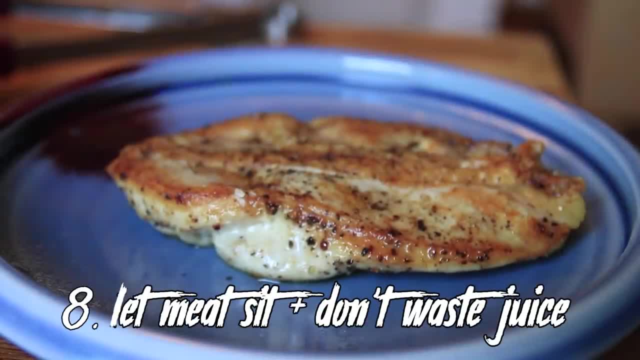 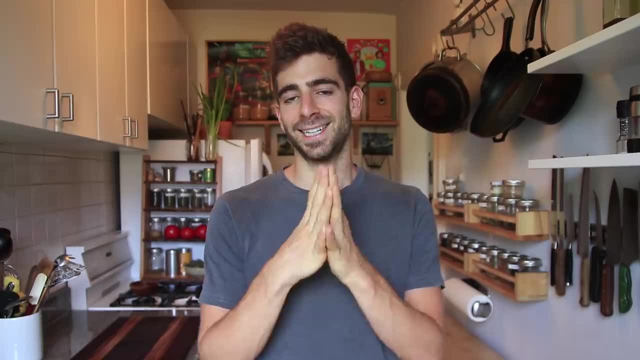 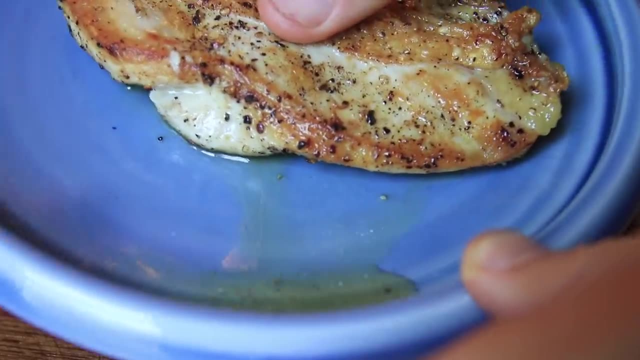 cook point. Tip number eight is a two-parter One. make sure you let the meat sit for at least 10 minutes. It's going to reabsorb those juices and stay nice and juicy. And the other one is if you get any juice that separates from the meat just like this, and that's normally going to happen. 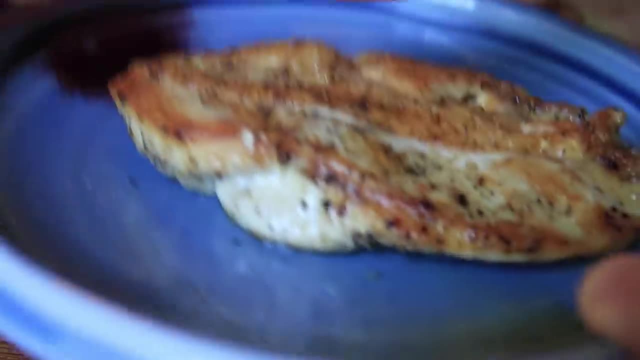 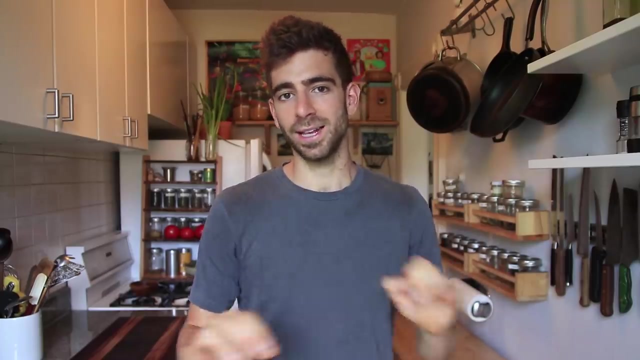 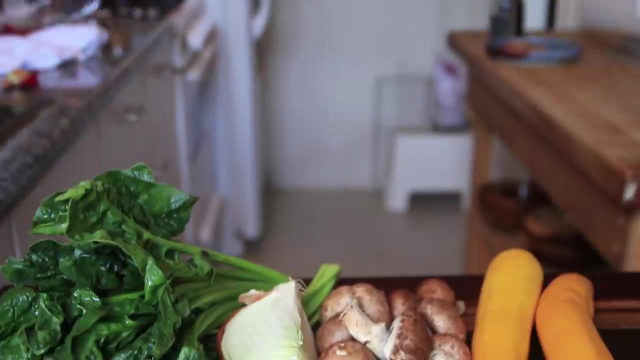 with meat. After a few minutes some of it will seep out. Make sure you do not get rid of that juice. That is extra flavor. You do not want to leave any meat juice behind, So save that and you can use that in your dish later, which you will see coming up soon. Moving on to the veggies and 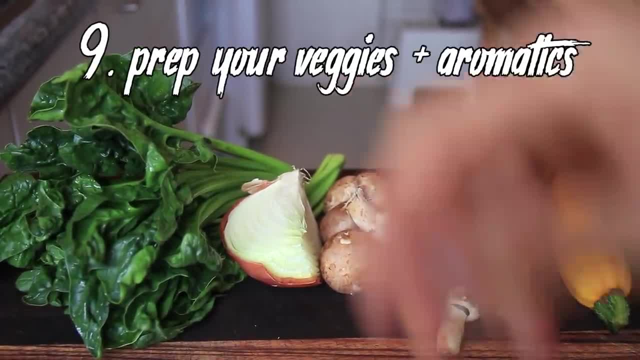 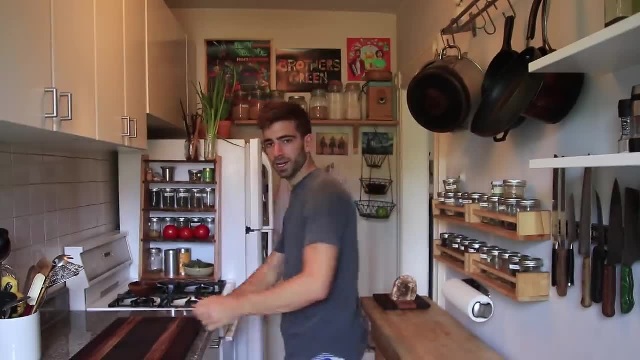 tip number nine is prepping everything before you actually cook, which is so important. If you're cooking, you're going to want to make sure that you're prepping everything before you cook. Prepping is really important, especially when you're dealing with high heat cooking, because you 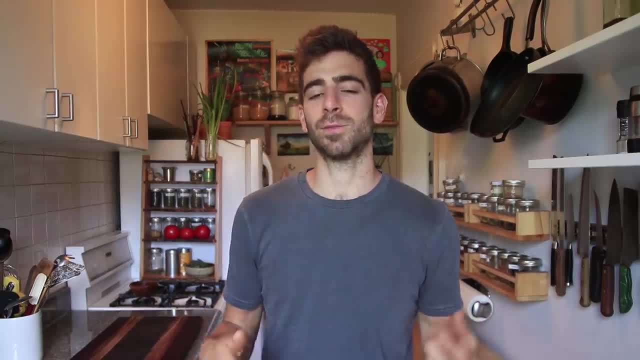 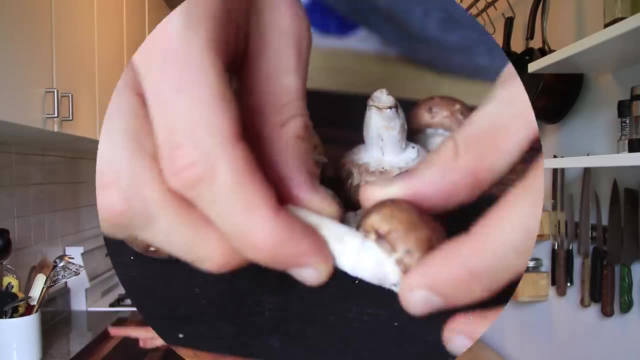 don't want to be cooking and cutting all the time. I used to do that when I was younger and things got a little out of control, And I still do that from time to time when I'm lazy. It's not the end of the world, But if you want perfection with your food, it's much easier if everything is prepped. 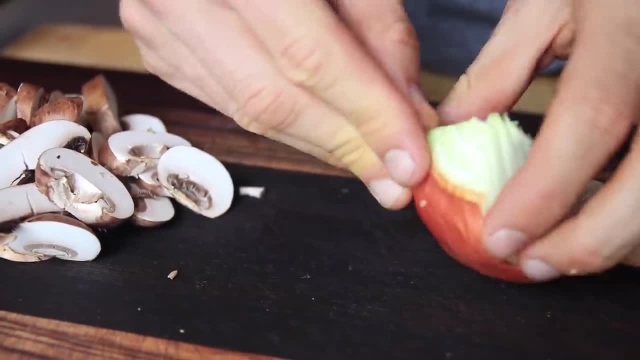 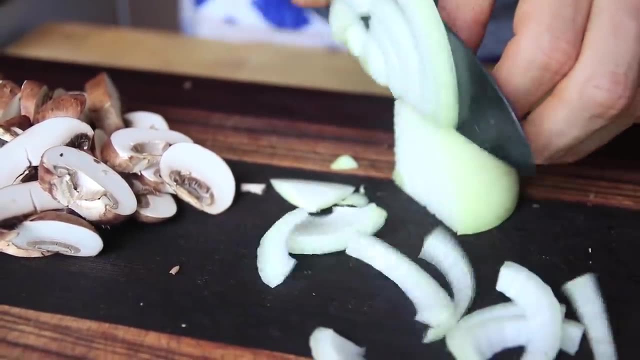 out. So here are the veggies we are using with our stir fry and we are going to prep all of this stuff. So we're going to start with the onion and we're going to chop it up. So you're going to want to be cutting and chopping it up how you like it. We've got the mushrooms we're going to give. 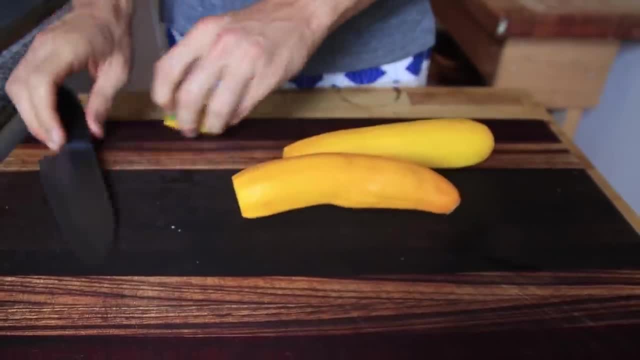 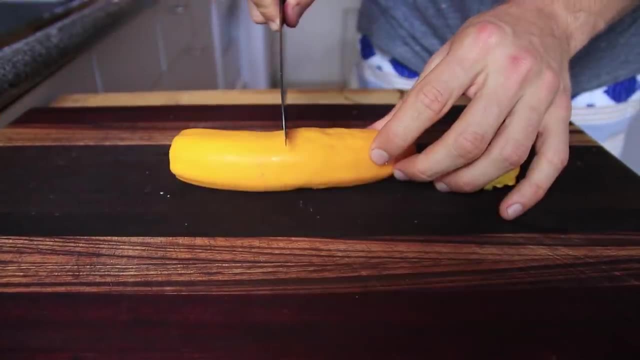 those a chop. I've got this little piece of onion. I'm going to chop that up as well. Here's a quick little bonus tip: when you're cutting zucchini, If you're having trouble getting even pieces because it's uneven like that, just cut it where it's uneven. Now you have two pieces that are a little. 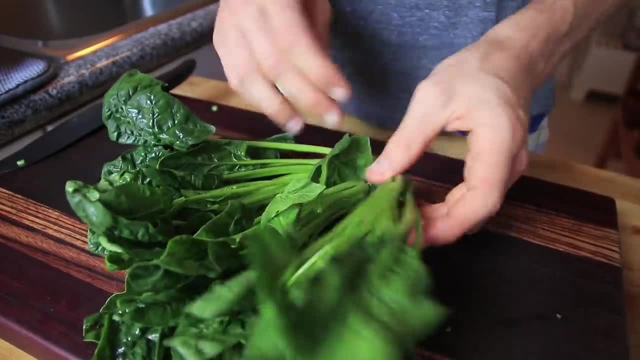 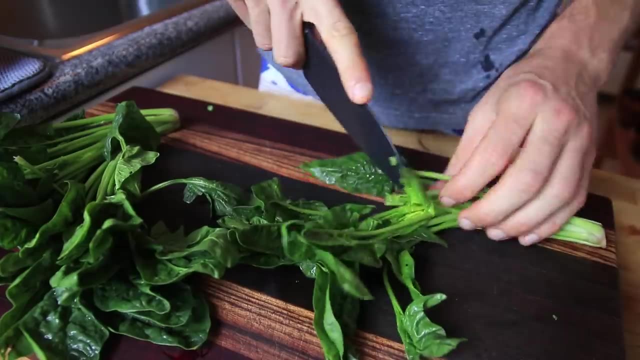 more straight and that will help with your actual cutting. And it's got the leaf. Sometimes the stem isn't going to come with it, it's going to be already pre-chopped. But if it comes like this, you can just chop that off because we've got the delicate. 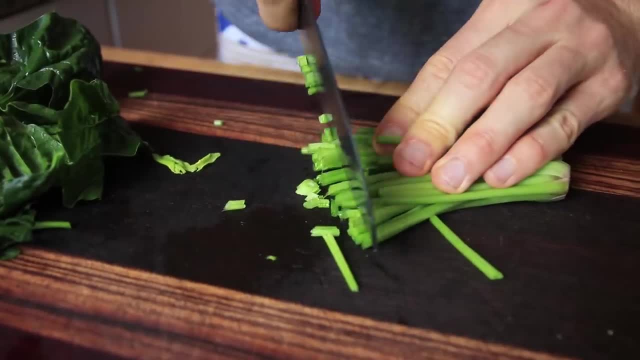 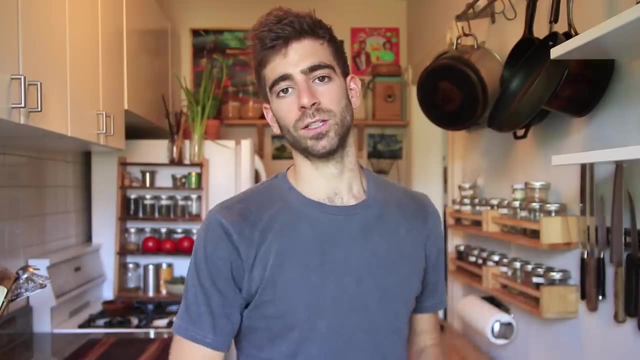 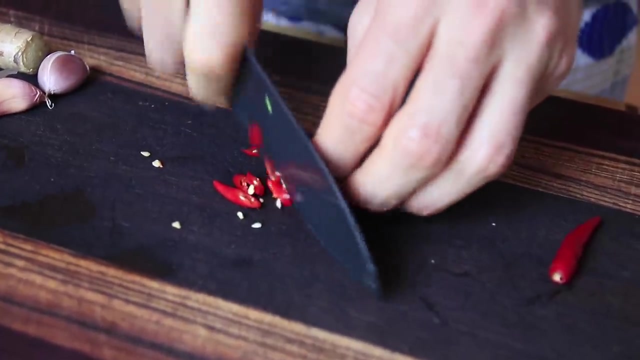 leaf, which is going to cook differently than the stem, And I'm actually going to put the stem with the aromatics. So we're going to wash that spinach, we're going to get all those veggies prepped, then I'm going to move on to cutting the aromatics. For this dish we've got a little bit of chili. 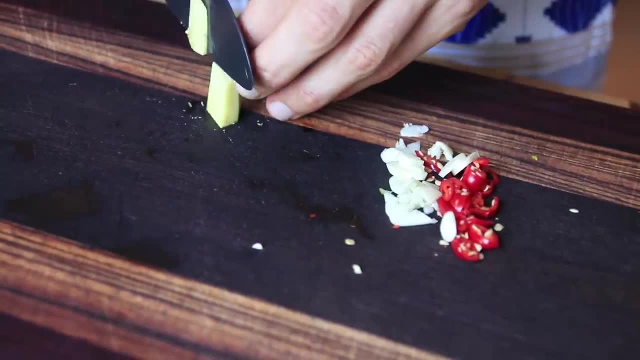 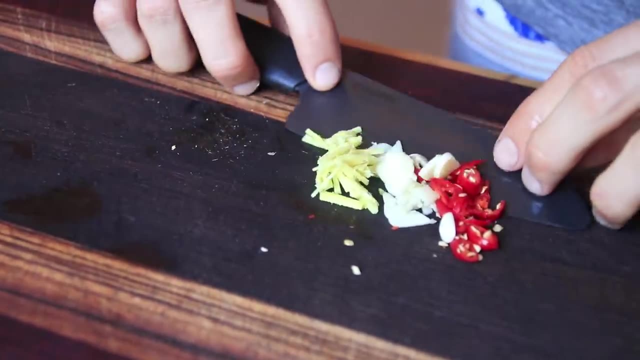 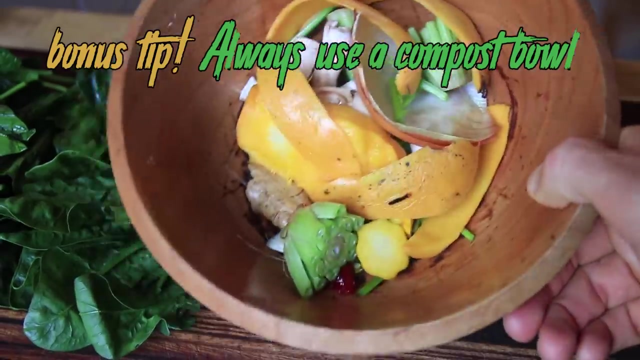 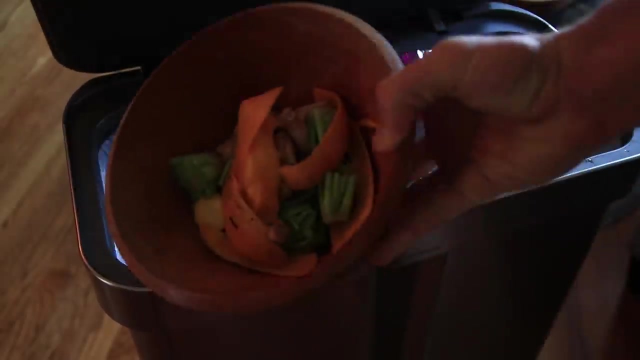 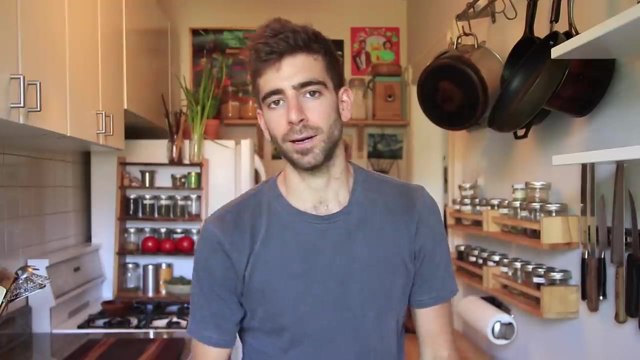